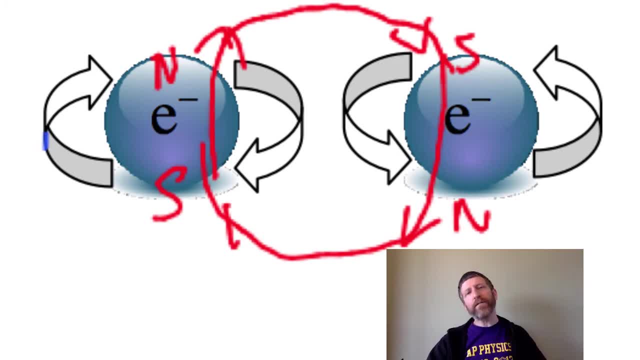 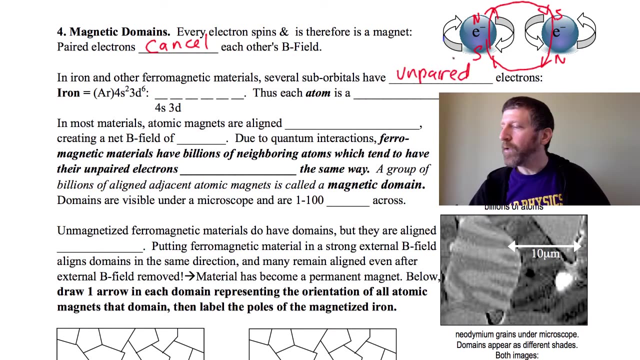 there. If you have paired electrons, you don't really have a strong B field. You have basically nothing because they cancel each other's B field. However, in iron and other ferromagnetic materials, several sub orbitals have unpaired electrons. Here's an example. Now you may have done this. 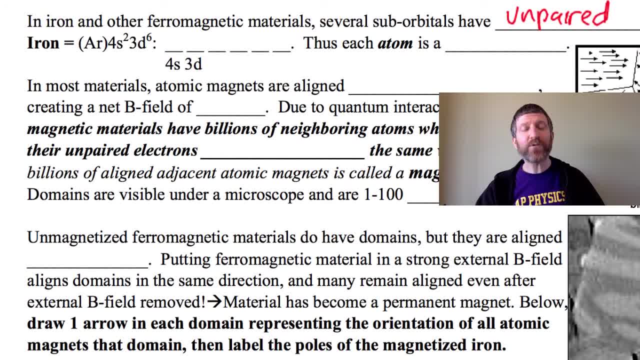 in chemistry, where you do these little up and down arrows, What you're actually drawing- although you didn't know- was the magnetic polarity of those electrons. For example, in iron we have va argon core, but then we add 4s2 and 3d6. So that means that all you got to do is 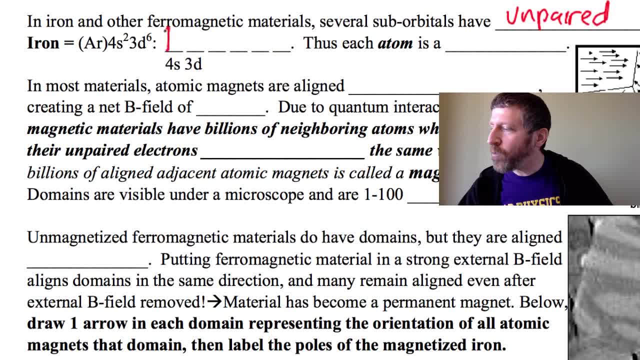 you first fill in the 4s shell, then spin up. the north pole of that electronic magnet is pointed up, then spin down. So we fill those in first, then we start filling in the 3d orbital with ups, spin-up, north pole, up, north pole up. 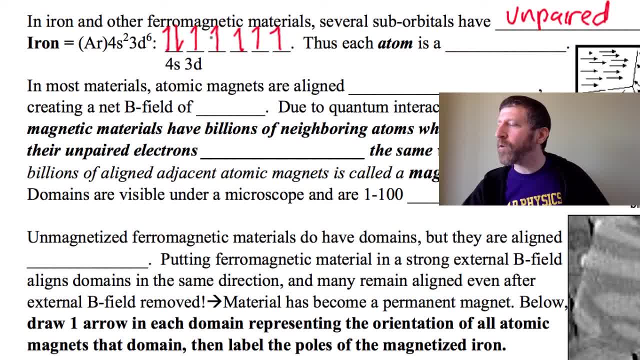 four and five, but then we have another one that we have to do, spin down right there. So you will notice that several of these electrons are unpaired. All these right over there have no pair. So every atom is a magnet, Every single atom of. 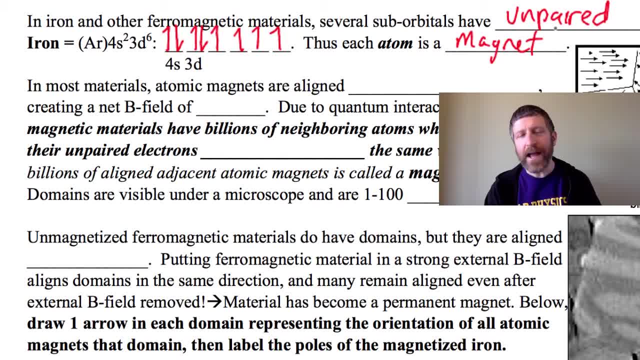 iron is a magnet. Now any, any material that's got unpaired electrons exhibits what's called paramagnetism, which is a weak magnetic effect, but certain things like iron, nickel and cobalt have ferromagnetism, which is an even more powerful magnetism. It has to do with what we're talking about now: domains Now. 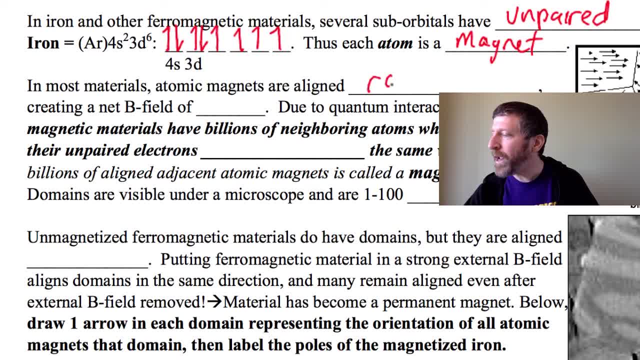 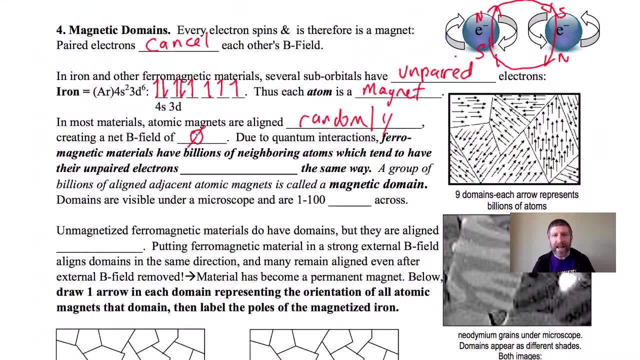 in most materials, atomic magnets are aligned randomly and that's what happens in paramagnetism. Every atom is a magnet, but if it's got unpaired orbitals. but they tend to align randomly, creating a net B field of zero. Now, due to quantum mechanical interactions, some materials- nickel, iron- 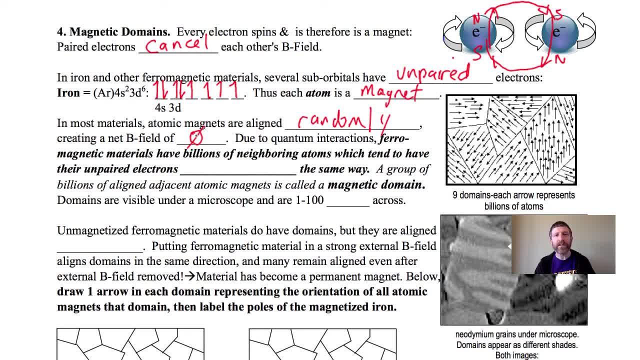 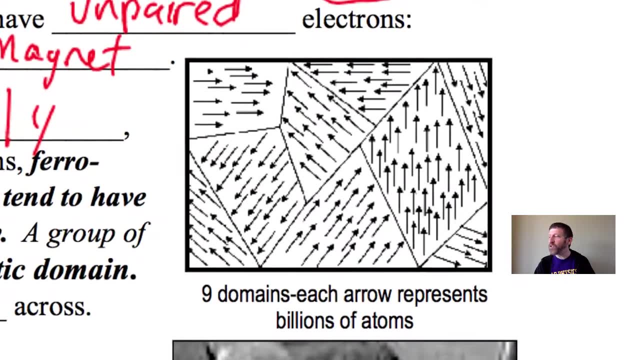 and cobalt to be specific, are ferromagnetic materials, and what they have is billions of neighboring atoms which tend to have their unpaired electrons aligned in the same direction. A group of billions of aligned adjacent atoms that are atomic magnets is called a magnetic domain, and in this picture, 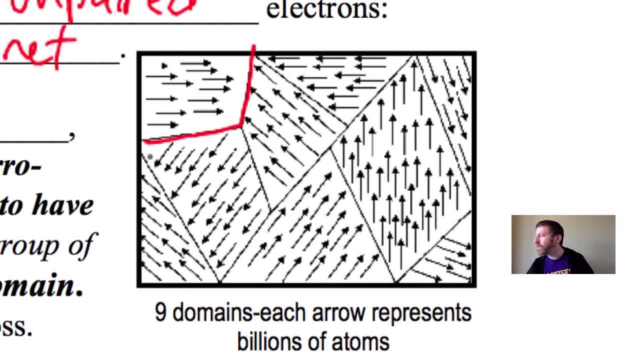 right here. every one of these sections here is a magnetic domain. Each one of these sections has billions of aligned atomic magnets. I'm outlining the domains Now. each one of these arrows, each one of these individual arrows, like this one and this one and that one, those each represent billions of atoms. So we're. 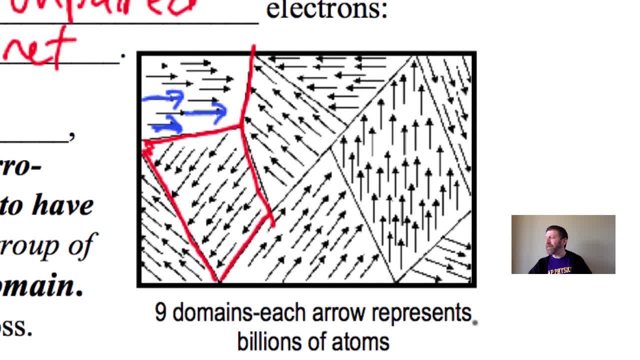 talking about many billions of atoms. This drawing right here has nine different domains and each arrow in that domain represents billions of atoms. So a group of billions of atoms that are aligned magnetically- they are aligned adjacent atomic magnets- is called a magnetic domain. So here's another domain. 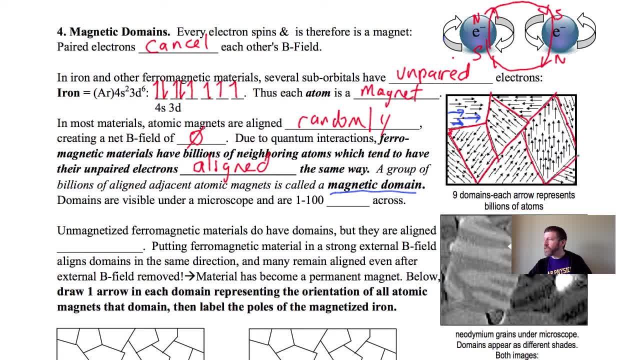 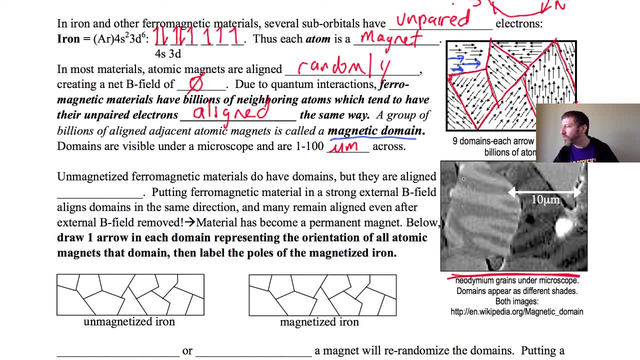 here's another domain. here's another domain, so you can see these domains. Now these are visible under a microscope. They're typically like 1 to 100 micrometers across. Here's a picture right here here. this right here is an actual picture. What you see as a different color right in there. 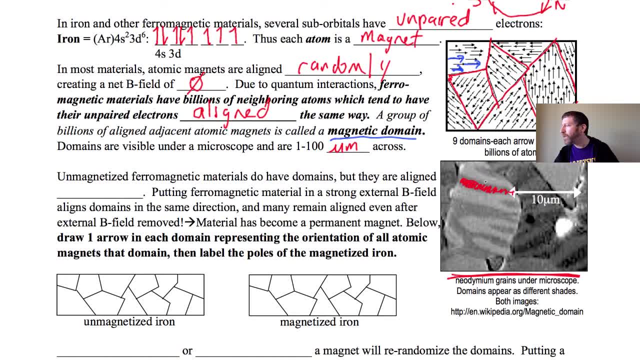 that is all one domain right in there And you have another domain right here and it's kind of shaped like that: Here's another domain right there. Anywhere you see a different color, that's a domain, a section of atomic magnets that are all aligned the same way. So that's what we're. 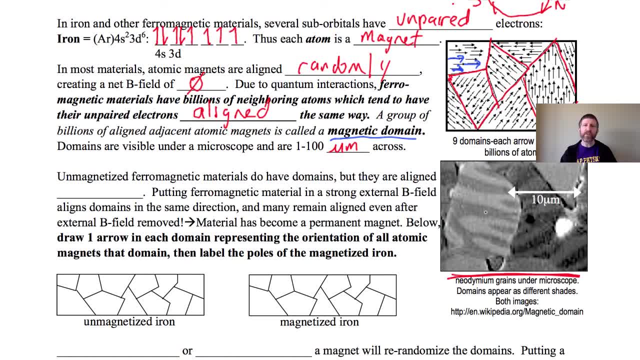 looking at right there And this length right there is 10 micrometers, so you can see how big the domains are. Unmagnetized ferromagnetic materials. they do have domains, but the domains are aligned randomly. In other words, let's draw a picture of this, For example: here's unmagnetized 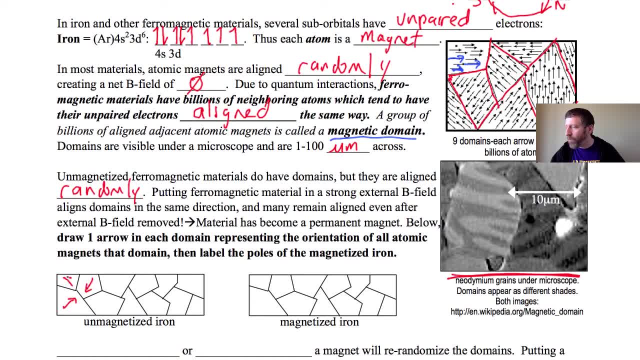 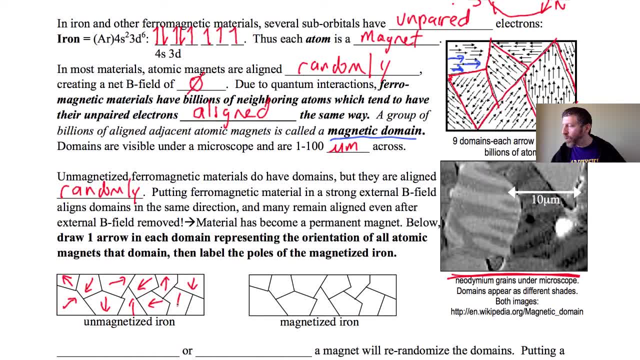 every domain with one arrow showing how the billions of magnets are. atomic magnets are aligned Here. in this picture up here, every arrow represents billions of atoms. In this picture right here, every arrow represents a single domain with its atomic magnets aligned in the direction. 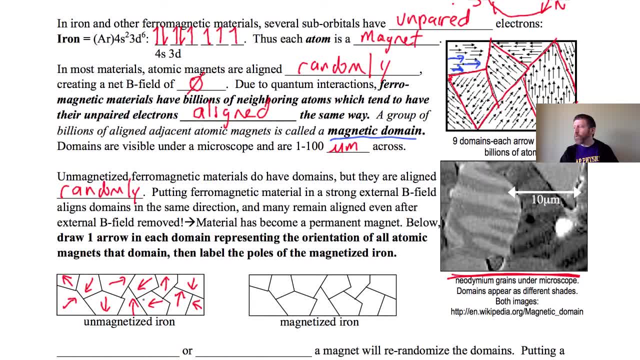 shown here. So what you do is, if you put a ferromagnetic material in a strong external B field, it aligns the domains in the same direction and many will remain aligned even after the external B field is removed. Here's a really cool applet that shows exactly that. So what we have here is a ferromagnetic 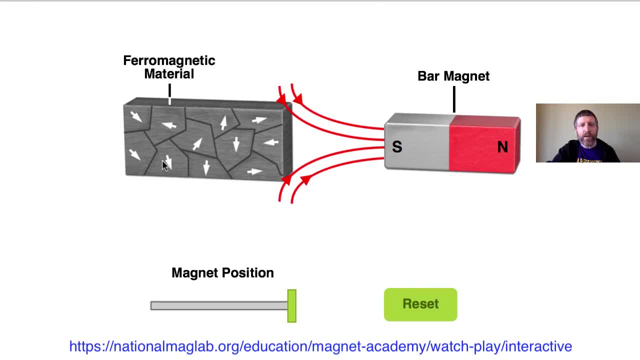 material and this represents the alignment or the orientation of each of the domains. Notice, they're aligned very randomly. What I'm going to do is I'm going to take this bar magnet which will provide an external magnetic field to this ferromagnetic material. I'm going to move the 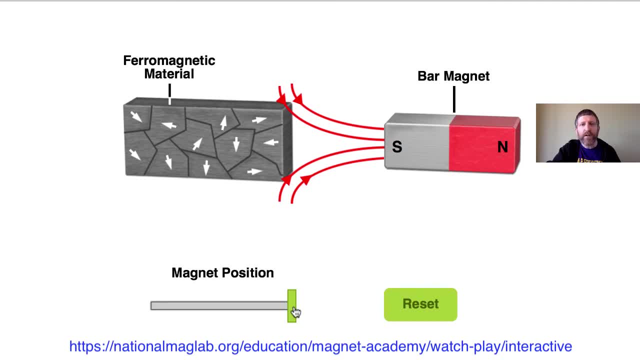 bar magnet close. Watch what happens to the alignment of those domains. when I bring this close, Notice that they're starting to spin and really what happens is the domains that are aligned with it actually become bigger. They absorb more atoms at their edges and 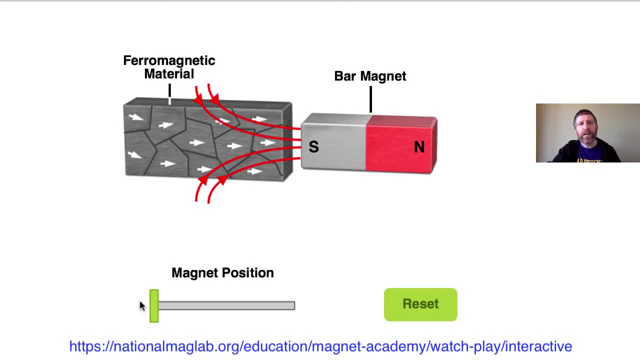 the domains that are not aligned get smaller, but what you end up with is the same thing in either situation. All these domains are aligning with this external B field and the internal magnetic field And even when I pull away the permanent magnet, those domains 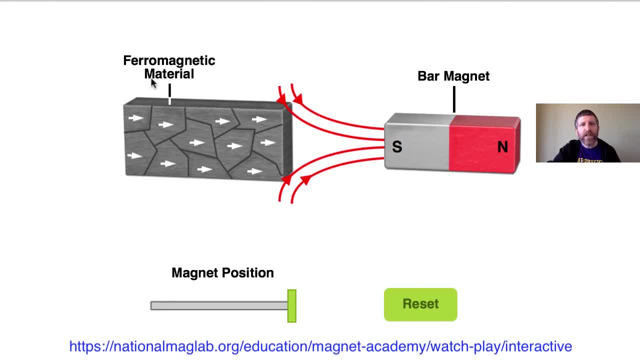 stay aligned. so now what I have right here? this thing is now a new permanent magnet. Now if I shake or heat this ferromagnetic material, or slam it really on the ground, or heat it to what is called the Curie temperature, those get re-randomized and it goes back to. 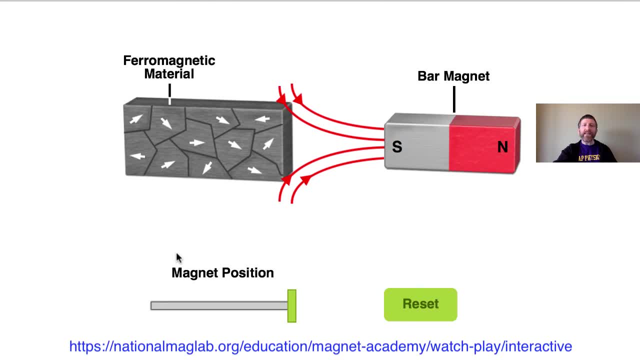 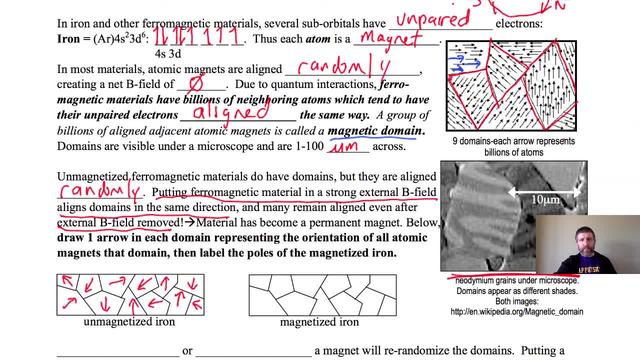 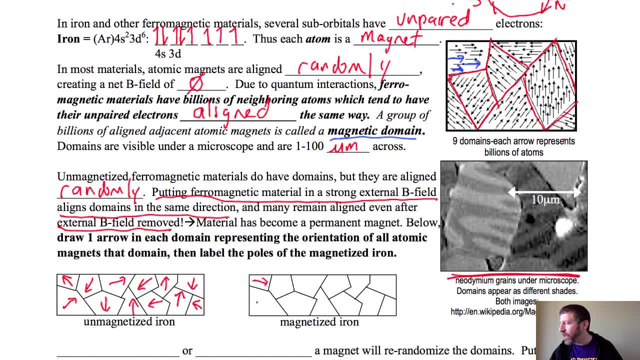 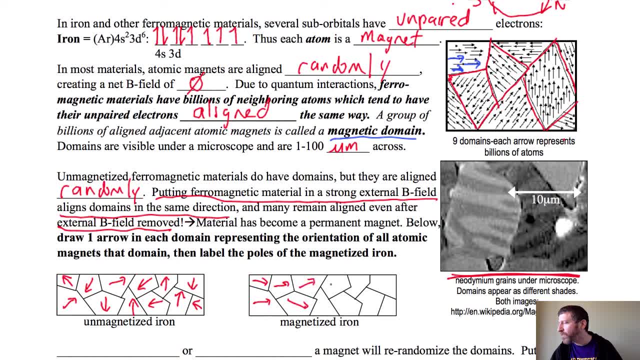 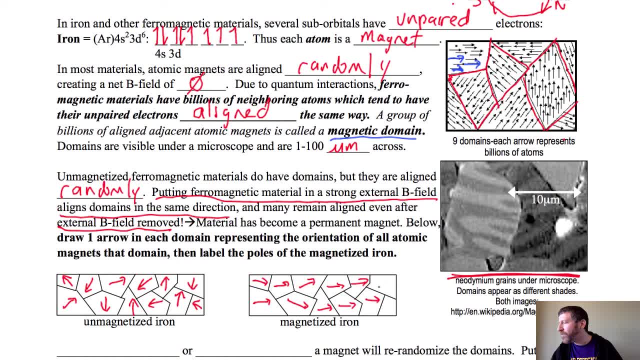 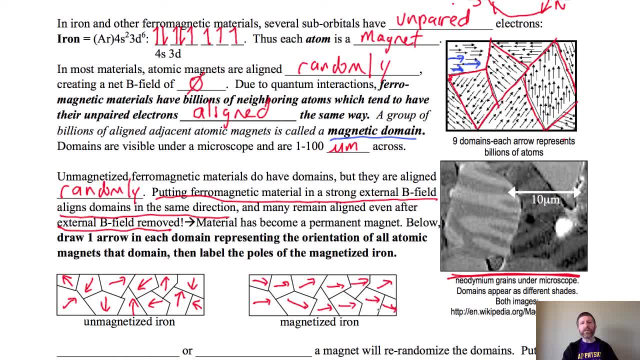